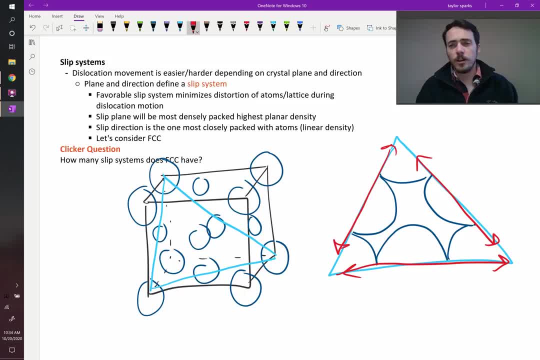 Right. So, taken together, if we could count up all of those directions in the crystal, we could count how many slip systems the FCC crystal has, Right? Well, what are those? They're these ones on this face right there. So if a cube has six faces and there is, you know, two different faces, 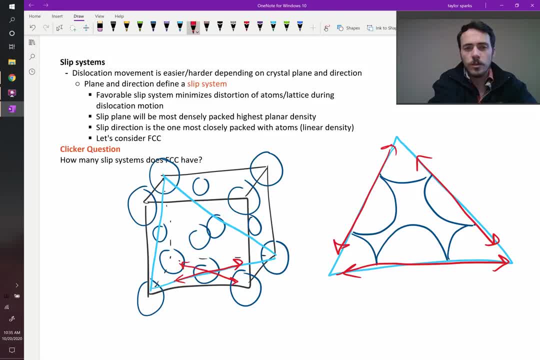 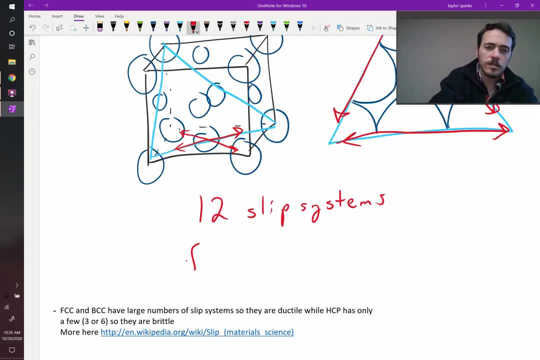 you know two diagonals per face, then there is 2 times 6, 12.. The FCC crystal would have 12 slip systems And again, that's because you've got six faces and two directions per face. Okay, So you end up with 12.. 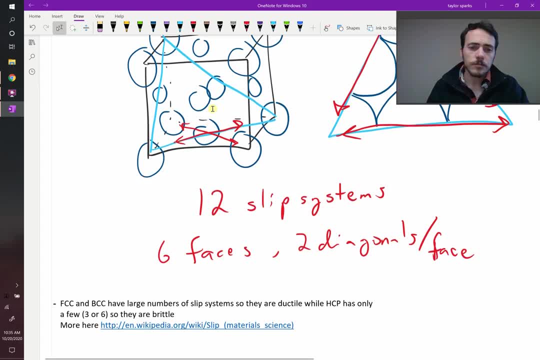 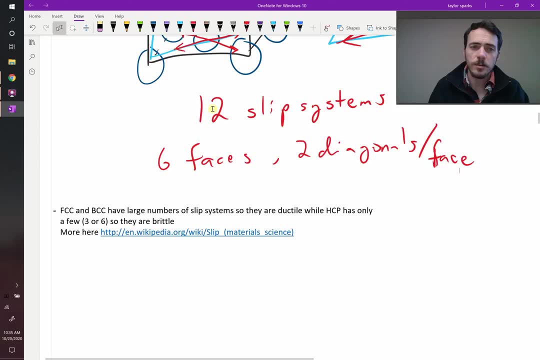 Right, You could do the same thing with BCC. You could count how many BCC has, or FCP, And what you'll find is that BCC and HCP and FCC have different numbers of slip systems. In fact, HCP has a number of slip systems. 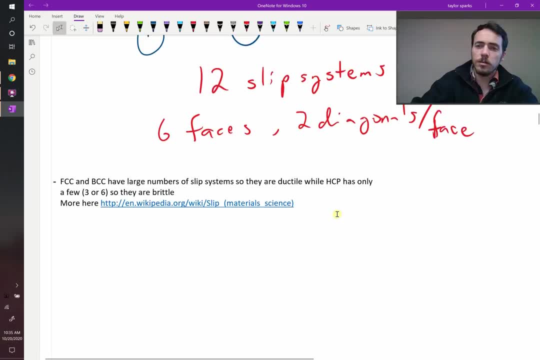 HCP only has three or six. It's along the basal plane Right. These atoms are located along this basal plane. where you have your atoms located like this, You basically get your slip systems in these directions And since it only has three or six, depending on how you count these, 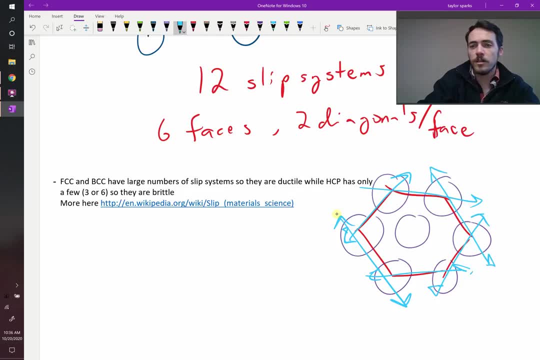 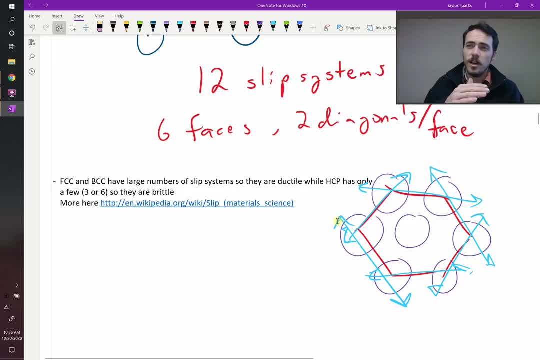 because it has fewer slip systems. So when you go to strain this thing, it's just fewer combinations of the ways the atoms can move in order to make it actually slide past one another, Okay, And therefore they end up being more brittle. 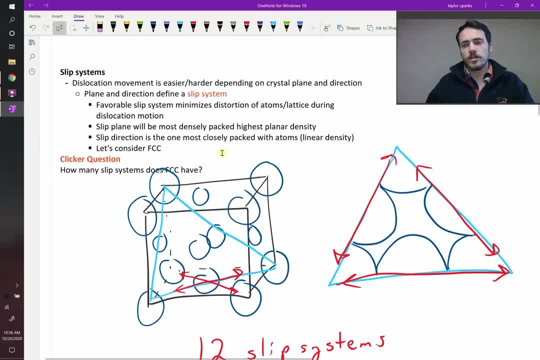 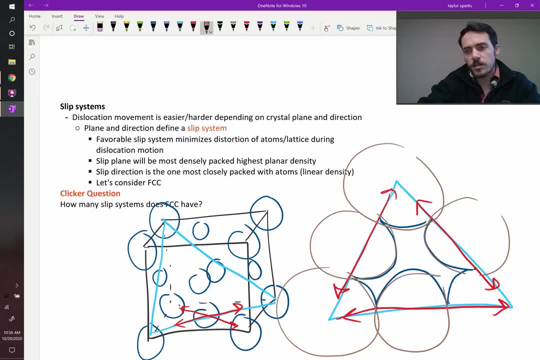 Now what do we mean? slide past each other? Take a look at this, If you were to strain this thing. literally, these atoms here and these atoms over here have to slide past one another. So as they slide past one another, we know that there's going to be an activation energy, right? 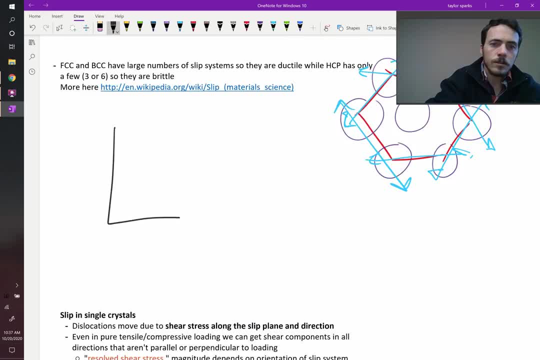 If you were to plot it, it would look like this: right, The energy as a function of distance, X. right, It's going to start out at some low point and you're going to have to overcome an activation energy and then get to another point.